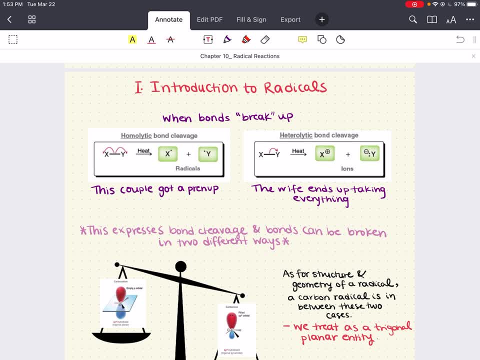 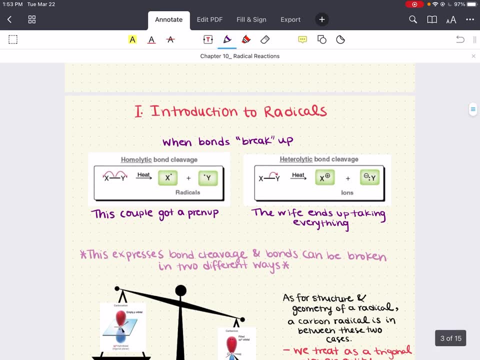 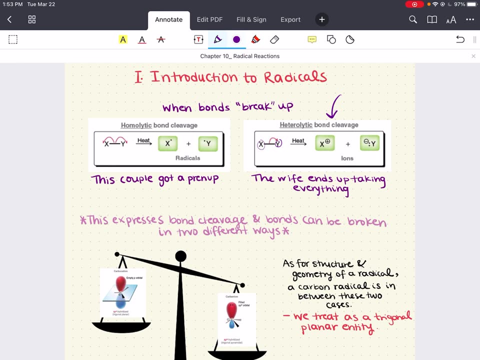 are taken by one of the atoms participating in the bond, This is going to result in ion formation. as a consequence, We could take a look here: Heterolytic bond cleavage. You have this bond between atom X and Y. When this bond breaks only one of these atoms, 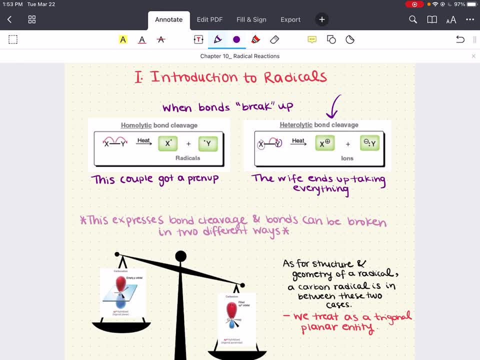 is going to take the electrons that make up this bond. That's Y. So Y takes both of the electrons that make up that bond. That results in a negative charge for atom Y and it results in a positive charge for atom X, because it has, because atom X has lost an electron total and atom Y has gained. 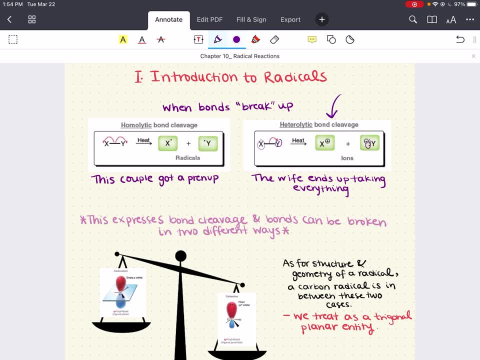 an extra electron, Hence the charge associated with X and Y and how heterolytic bond cleavage results in this ion formation. In homolytic bond cleavage each atom in the bond gets a single electron, All right, So they share it fairly and this forms radicals as a consequence. You can 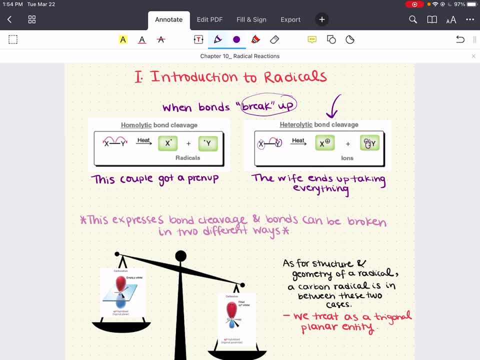 think of this as well. when the bonds break up, what happens In heterolytic bond cleavage? the wife ends up taking everything All right. In a homolytic bond cleavage, this couple, they got a prenup. They get what they came in with. 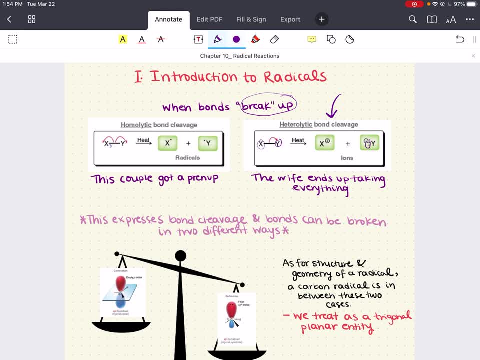 All right, And so every atom's electron participating in the bond goes back to that atom. All right, Fantastic. Now, as you notice, with homolytic bond cleavage right here, it's depicted through this single barbed arrow. It's not a full arrow, It's like half an arrow. 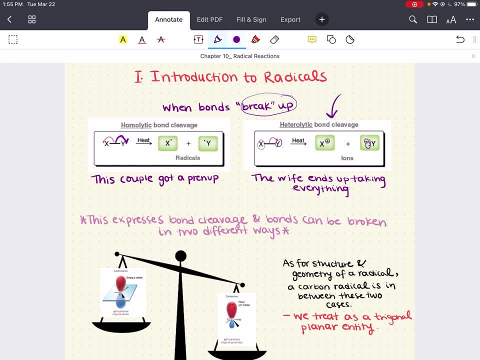 All right, These are. this is called fish hook and this shows the motion of one electron. We're going to be using this arrows a lot in our discussion today of radicals, So it's good to make note of it and to understand that a full arrow depicts the movement of two electrons and a half. 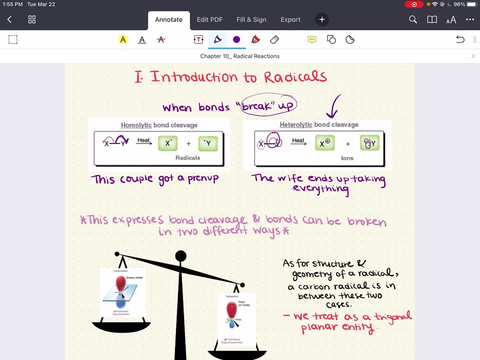 arrow. this fish hook single barbed arrow depicts the motion of one electron. Now, in order to understand the structure and geometry of a radical, let's look first at the geometry of a carbocation versus the geometry of a electron. So let's look at the geometry of a carbocation versus the geometry. 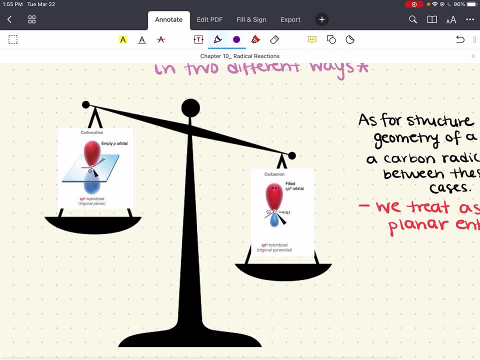 of a carbon anion In a carbocation. the carbocation is an sp2 hybridized and it has a trigonal planar geometry. All right, So it's sp2 hybridized with trigonal planar geometry. A carbon anion is going to be sp3 hybridized and it's going to have a trigonal pyramidal. 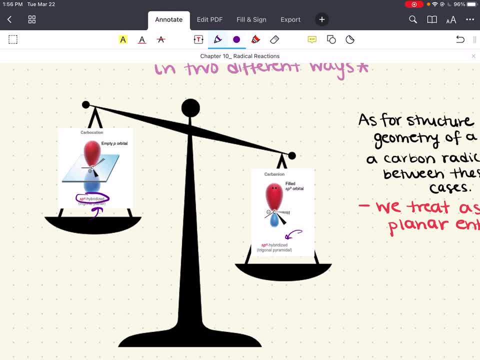 geometry. The difference in geometry is that it's going to have a trigonal. pyramidal geometry Obviously results from the difference in the number of non-bonding electrons. A carbon radical is going to be in between these two cases in terms of non-bonding electrons. All right, So in a 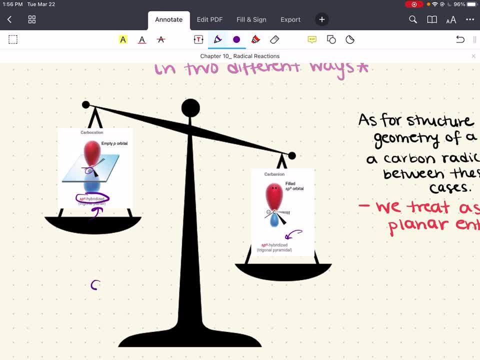 carbocation. all right, we have a carbocation because the carbon has three bonds, There's no lone pairs, Okay, And it doesn't meet its octet, Hence why it has that positive charge. All right, This is sp2 hybridized Now in a carbon anion. the carbon has three bonds and it has a lone pair. 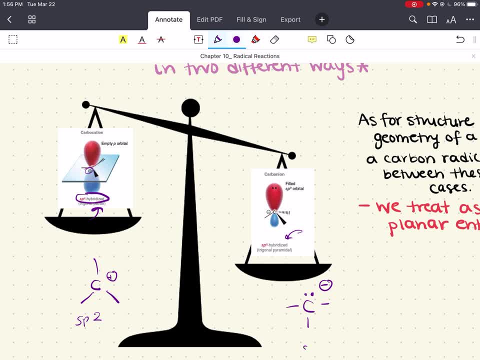 Hence the negative charge on there. This is sp3 hybridized. Now for carbocation: three bonds, no lone pairs, which is why it's trigonal planar. Carbon anion: three bonds, one lone pair, All right. Hence why it's trigonal pyramidal. 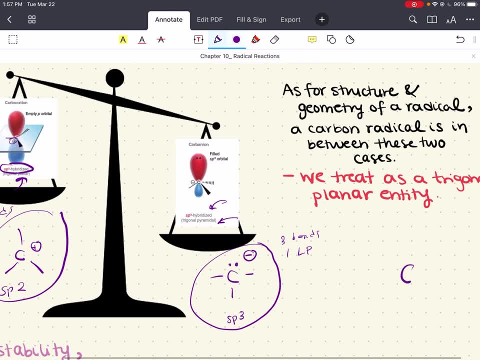 Now a carbon radical. let's draw this. A carbon radical will be somewhere in between. Carbon has three bonds, one electron, not a lone pair, just one electron. All right, Now it's between the two cases for carbocation and carbon anion in terms of non-bonding electrons. 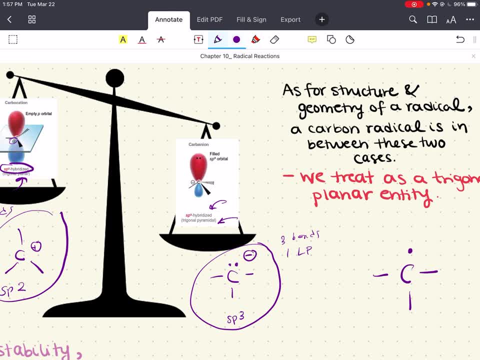 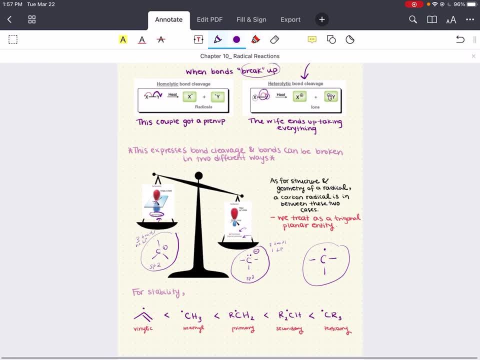 But regardless, what you should know is that it's still treated as a trigonal planar Entity. All right, So make sure you note that now the order of stability for carbon radicals follows this hierarchy right here Now. this is very important to keep in mind. All right From. 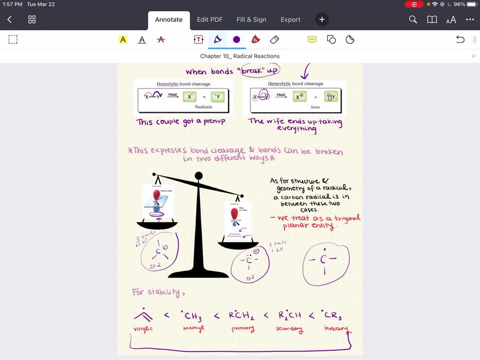 least stable to most stable, with this end being least stable, this end being most stable. We start off with a Vinlick position. Whenever you have a radical at the Vinlick position, that means at the location of the double bond, As you see here, this is gonna be the least stable form of a carbon radical. 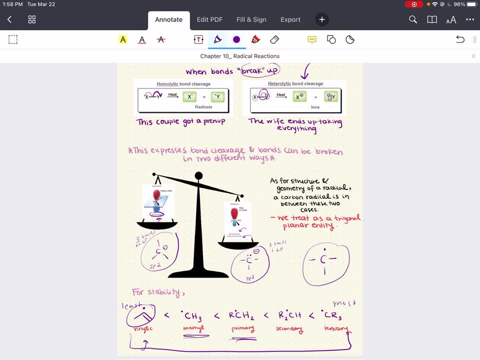 Next up is a methyl, All right. Then a primary- uh uh uh. carbon entity. secondary and then tertiary, where tertiary is the most stable, Now. Now, the reason for this order of carbon radical stability is based on hyperconjugation. Alkyl groups are capable of stabilizing the unpaired electrons through delocalization effects, which is why, as you add R groups- whether they be alkyl or acyl groups- to carbon radicals, you result in this higher stability in the carbon radicals. 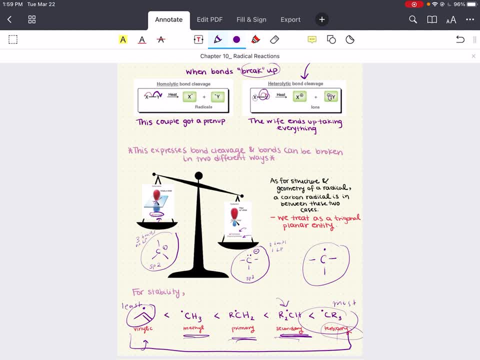 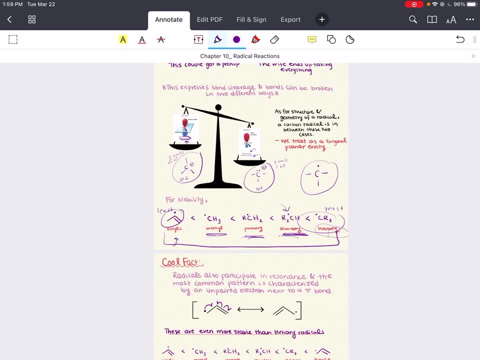 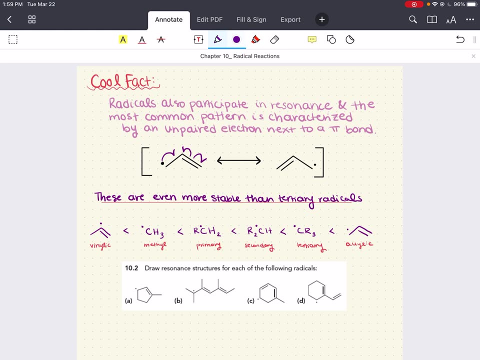 And that is because, again, alkyl groups are capable of stabilizing the unpaired electrons. Now, another thing about radicals is there are several patterns for drawing resonance structures of radicals. The vast majority of situations require only one pattern, and that pattern is characterized by an unpaired electron. 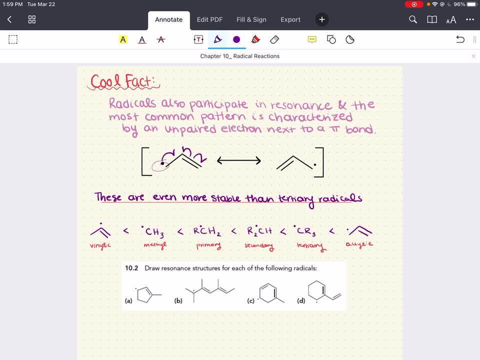 near a double bond or a pi bond. in general. It could be a triple bond too, So it is characterized as patterned by an unpaired electron next to a pi bond. So radicals also participate in resonance, and that is the most common pattern for radical resonance. 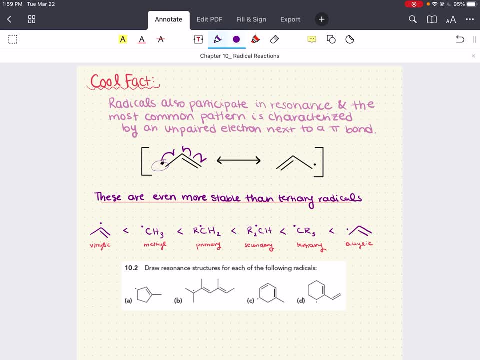 So what this means is, whenever you find the single electron near a double bond, it can participate in resonance and you can draw the resonance structures. Now, how do you appropriately draw this resonance structure? Well, starting off at the single electron you have using a fishhook arrow. 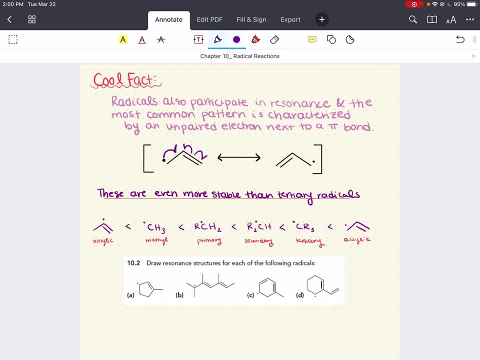 that electron will come to this bond along with one of the electrons of the double bond, And what happens now is we're going to form a double bond here, as you see, And that means that the other electron, The electron of the double bond, gets put at the end here. 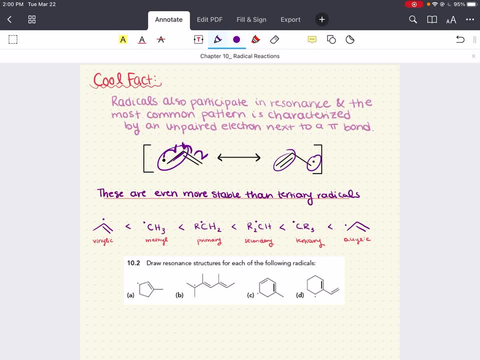 And so that's how you want to draw the resonance structures for carbon radicals. Now, a very important thing to know, and we're going to go back to our hierarchy of carbon radical stability, allelic radical positions. They are, in fact, more stable than tertiary radicals. 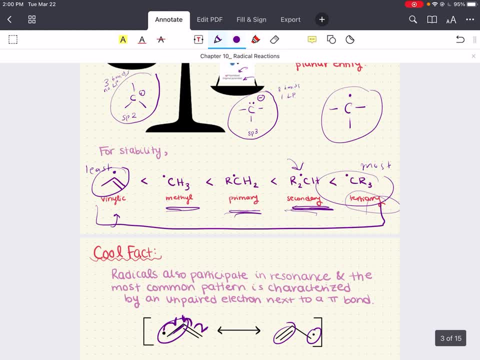 So we need to add that to the order of stability we have Here. we have, When we first introduced it, that our tertiary carbon radicals are the most stable. there is one thing that is more stable than a tertiary carbon radical. That is a allelic radical position. 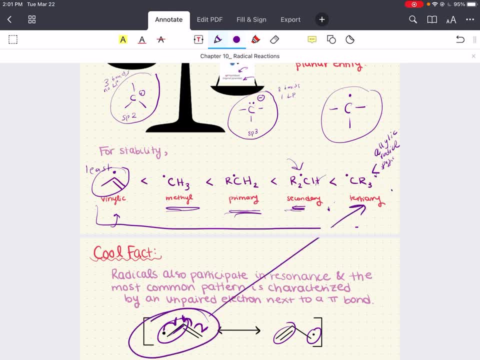 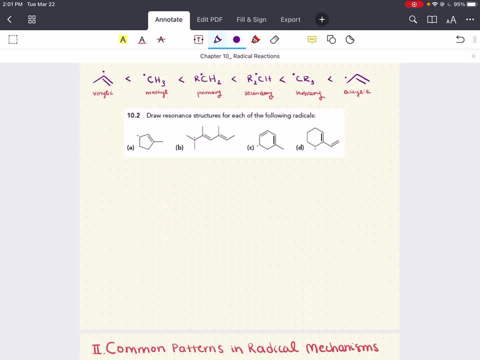 All right. So something like this would be more stable than a tertiary carbon radical. All right, Now let's do a practice problem or two to get the hang of drawing our fishhooks, Fishhook arrows, as well as drawing the resonance-stabilized structures for radicals. 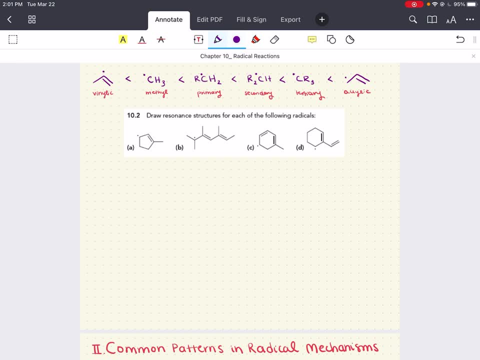 All right, So draw resonance structures for each of the following radicals. We're going to do A. All right, So let's make note. We have a single electron here. It's right next to a double bond. All right, We're going to use fishhook arrows to demonstrate the resonance structures of this molecule right here. 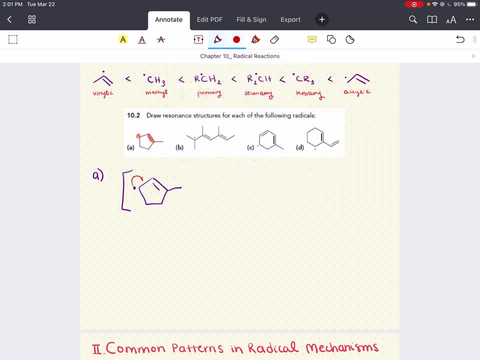 Well, if we have an electron, We have an electron right there. This single electron can come here along with one of the electrons of the double bond, and we're going to form a double bond here now. All right, There's still another electron in this double bond. 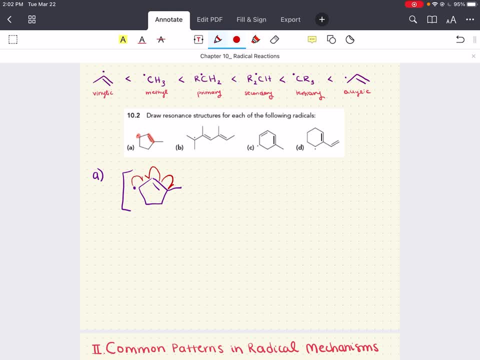 It's going to get dumped on the opposite end, And so what that means is our resonance structure, for this molecule is going to look something like this: Fantastic, Let's do B. All right, Here's B. Let's draw it out fully. 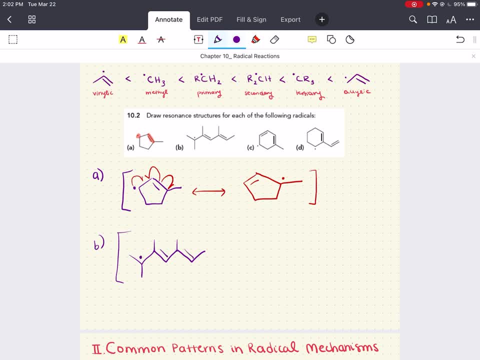 We have our lone electron right here. All right, We want to draw the resonance stabilized structures for this molecule. Here we have our single electron near a double bond. We're going to go ahead and draw that appropriately. The single electron will come here along with one electron from the double bond to form a new double bond here. 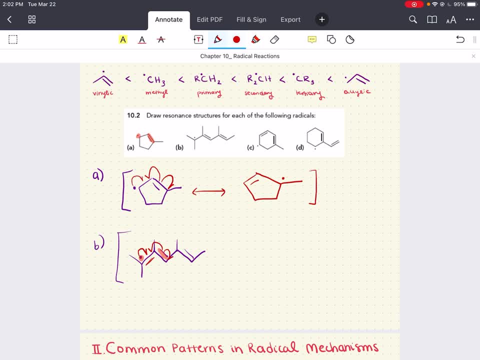 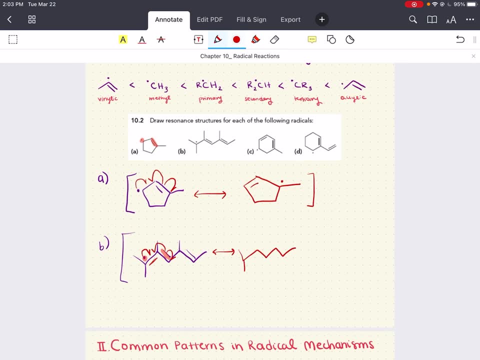 All right, But there's still a single electron from this double bond. It's going to get dumped. It's going to get dumped right there. What that means is we're going to have a resonance structure that looks like this: All right. 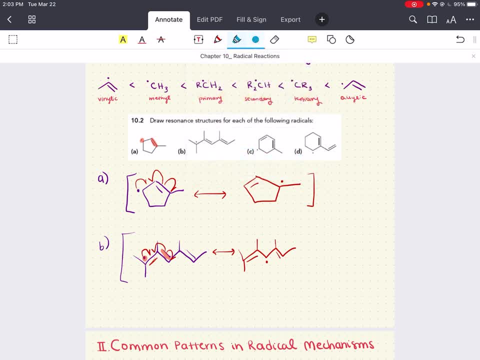 Well, we're not done yet, because- look at this Again- we have a single electron near a double bond, So let's continue to draw all the resonance structures for this molecule. Now this single electron will come here along with one of the electrons of the pi bond. 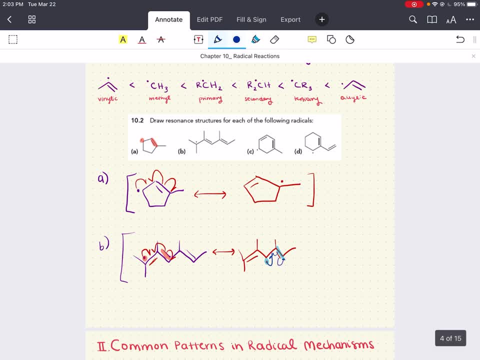 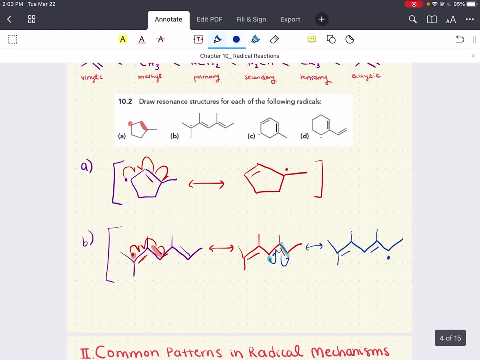 It's going to form a new double bond there, And that last electron will get dumped here. Fish hook arrows, don't forget. And so we get something that looks like this: Perfect. And this is the resonance structure for molecule B. 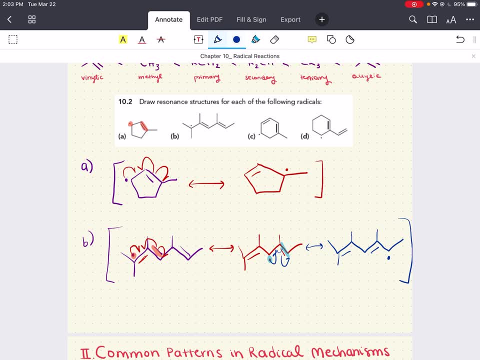 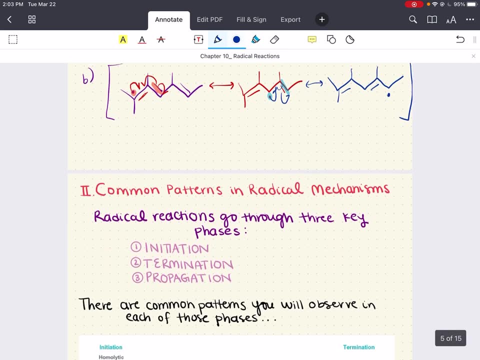 I'm going to let you attempt C and D. Let me know what you get in the comments below And if you need help, feel free to reach out to me. But next, what we want to discuss Are common patterns in radical reactions. 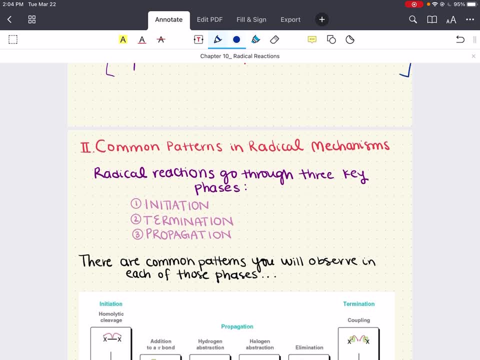 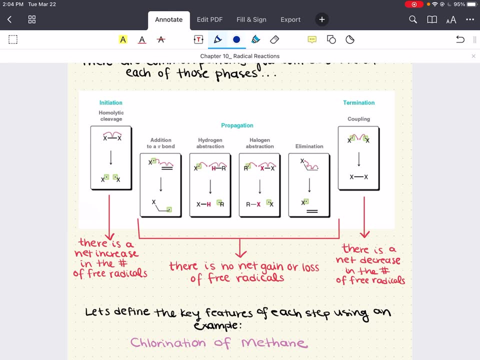 Now radical reactions go through three key phases. The first phase is initiation. Here there is a net increase in the number of free radicals. This phase is described essentially by the pattern of homolytic cleavage. All right, So initiation implies homolytic. 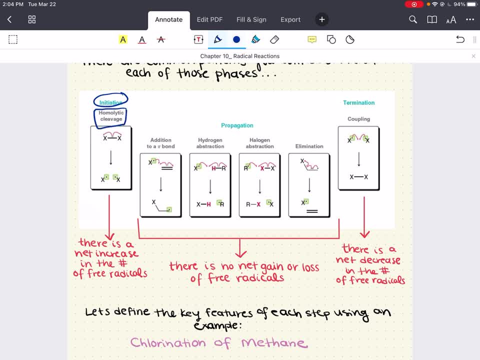 And here there is going to be a net increase in the number of free radicals. Also, note that free radical reactions. they require heat or light to be applied for the homolytic bond, cleavage, to occur. So in order for initiation, which is the first step of a radical mechanism, to occur, 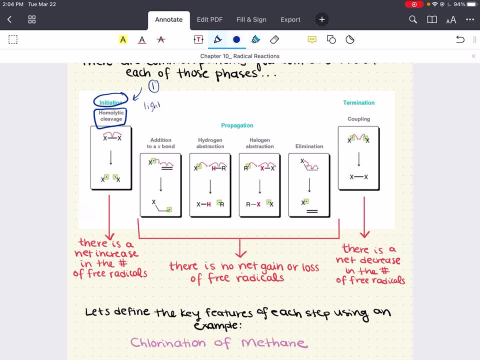 we're going to need to have light or heat to make it happen, To make this possible, All right. With light or heat, homolytic cleavage, which is an initiation process, will occur, And homolytic cleavage means that a bond between two atoms is going to get broken. 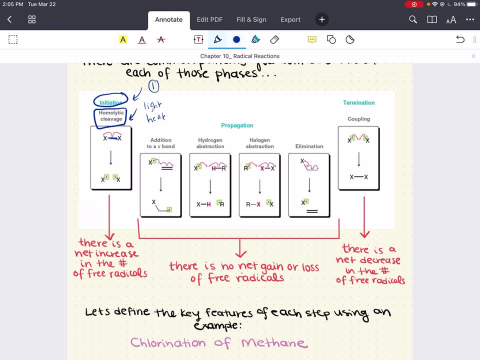 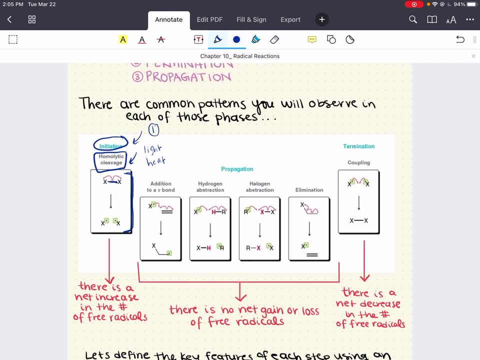 Where each atom leaves with a single electron, like you see demonstrated here, Fantastic. The second phase of radical mechanisms is propagation. In this step There's no net gain or loss of free radicals. The common patterns you're going to see in this phase are one of four. 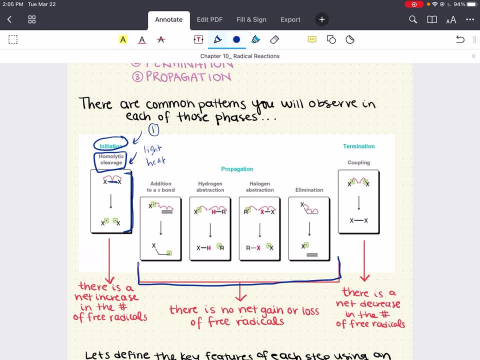 All right. One of four first common pattern you're going to see in the propagation phase is addition to a pi bond, where you, a radical, adds to a pi bond and thereby destroys the pi bond And in Its process, generates a new radical. 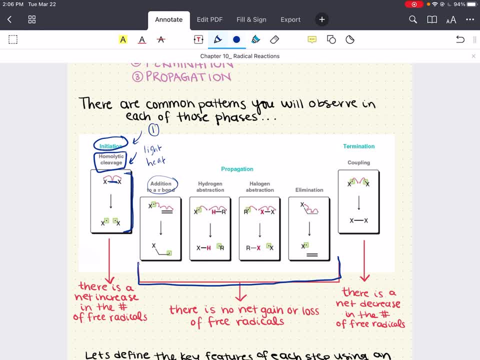 So addition to a pi bond is one common pattern you'll see in propagation. Another common pattern you'll see in propagation is hydrogen abstraction. here, As the name says, a radical can abstract a hydrogen atom from a compound And what this is going to do is going to generate a new radical. 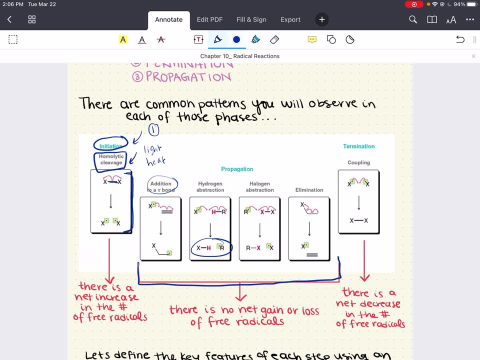 As you see here. another thing that can happen, Another common pattern in propagation. In propagation is halogen abstraction. This is just like hydrogen abstraction, but with halogens. So a radical can abstract the halogen atom from a compound and generate a new radical again, as you see here. 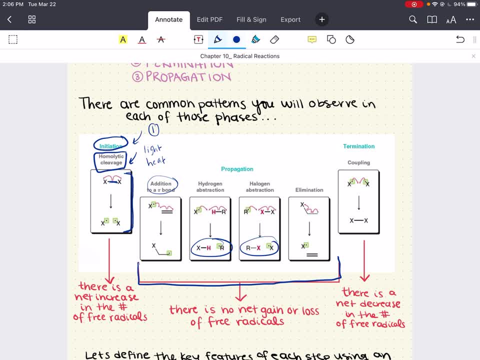 And the fourth common pattern you can see during propagation phase is elimination. What happens in elimination is a double bond forms between the alpha and beta position, And the beta position is It's cleaved, causing the compound to fragment into two pieces. So what you see here, what can happen, is the single bond can break off where the atom attached takes one electron, and then this radical electron as well as a one electron from this bond gang up to form a double bond. 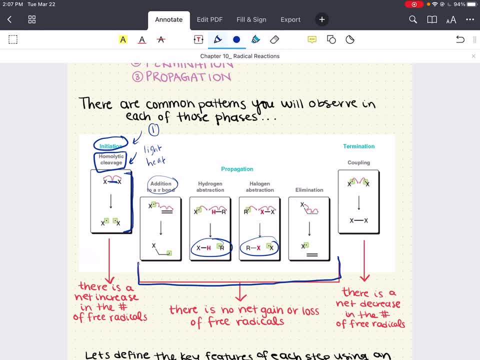 So a double bond is formed between the alpha and beta position And the beta position is cleaved- sorry, I drew this wrong- between the alpha. where the radical is, is the alpha and the beta position. All right. where the beta position is cleaved, that means cut off, causing the compound to fragment into two pieces. where you get a double bond for one. 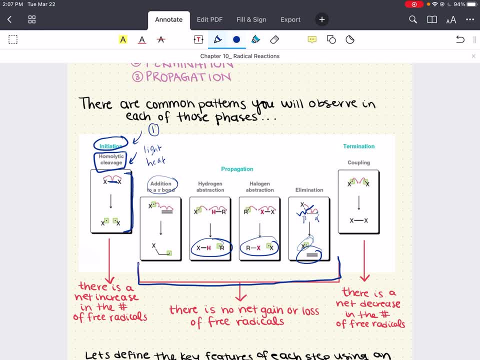 And then your X molecule that's attached there leaves as a radical. All right, the last phase is termination. In this step there is a net decrease in the number of free radicals. So in initiation there was a net increase in termination, which is your final step. 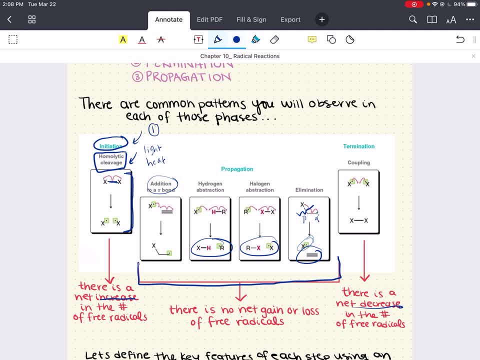 There is a net decrease in the number of free radicals, And the common pattern you're going to see for this step is coupling. Coupling is when two radicals join together to form a bond, All right, so it's the complete opposite of a homolytic cleavage. 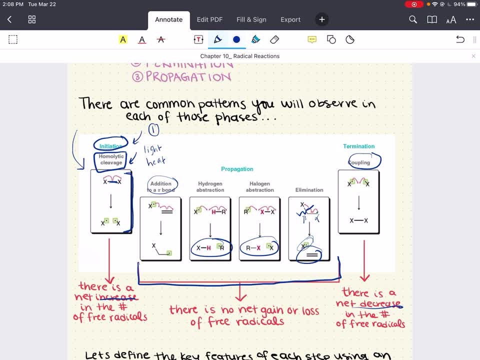 All right, you need homolytic cleavage for your initiation In the initiation phase. all right, you have a bond that breaks. all right, and each molecule gets one of those electrons. right, Like we said when A, when this bond couple breaks up, all right, they got a prenup, so each one leaves with an electron. 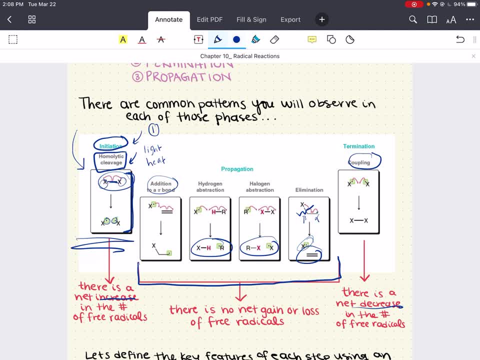 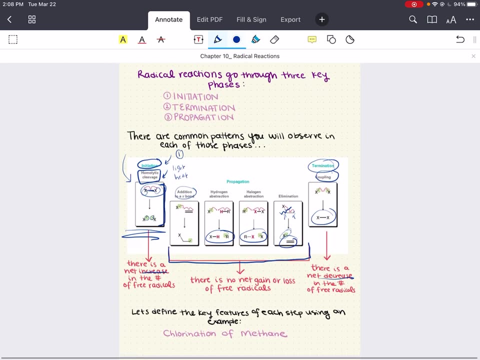 This initiates radical mechanisms. What ends it is termination when the couple gets back together again. all right, And we're going to see this in play, all right with an example, By talking about chlorination of methane. But before we get there, I want to say one thing about this intermediate step, the second phase of radical reactions, which is propagation. 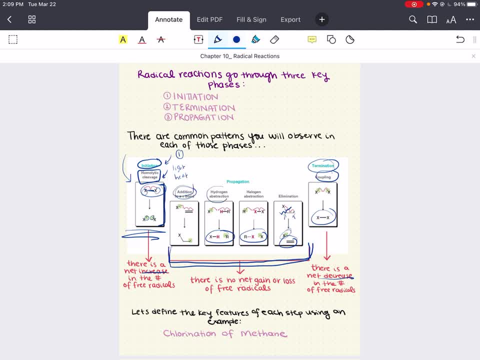 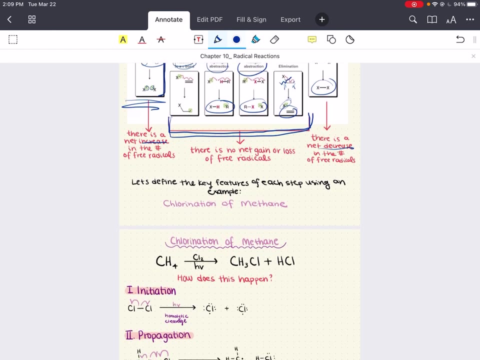 Here you can get several of these occurring, where the net reaction of all the steps that might occur during propagation add up to your ultimate reaction goal. And we're going to see that even. And we're going to see that even better when we do chlorination of methane, and we're going to do that now. 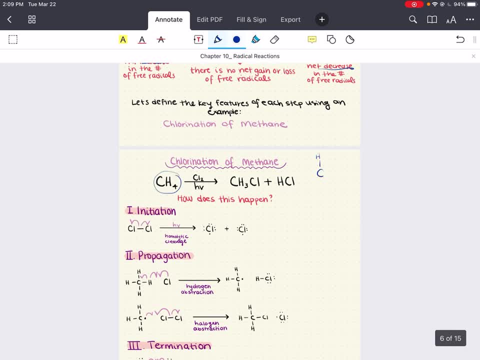 All right, so we have methane. This is what methane looks like, See, which is carbon, with four hydrogens attached to it. All right, we treat it with Cl2 and some light. all right, And what we get is this: gets converted to chloromethane. all right, where we have a hydrogen. 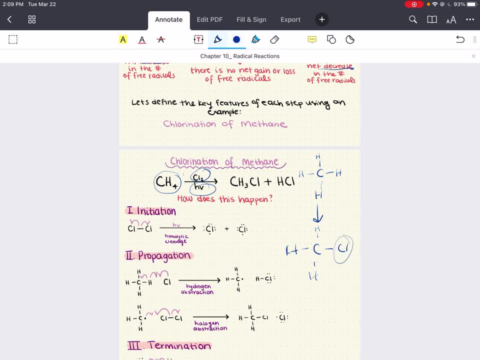 All right, That is replaced with a chlorine. all right, So when we have methane, we treat it with Cl2 and light. all right, We're going to replace one of the hydrogens with chlorine. How does this happen? Well, first step of a radical reaction is initiation. 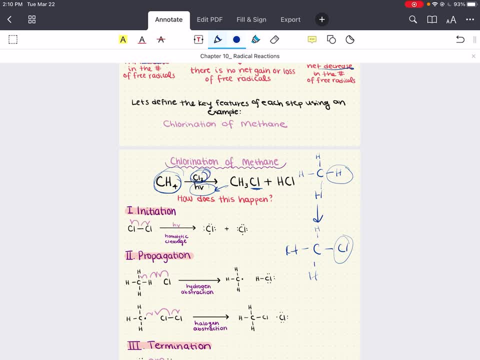 What happens is initiation is creation of radicals. We're going to need light or heat to promote this step, which we have, and we create chlorine radicals. So our first step, Our second step, is initiation. all right, The Cl2, along with light, causes homolytic cleavage, which is our initiation step. 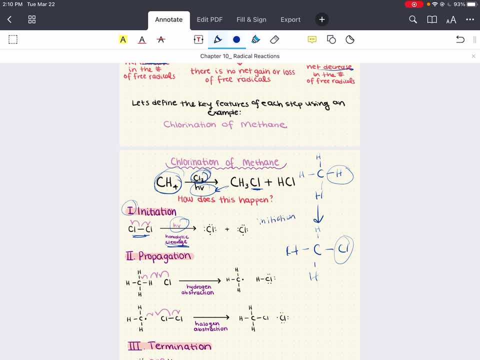 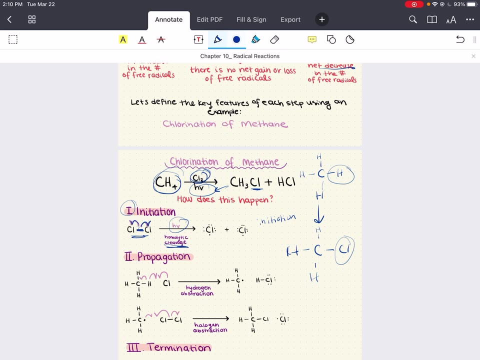 Remember, homolytic cleavage is associated with the first step of radical mechanisms initiation. So our Cl2 is treated with light, all right, It gets homolytically cleaved. What that means is this bond breaks and each chlorine gets an electron. all right. 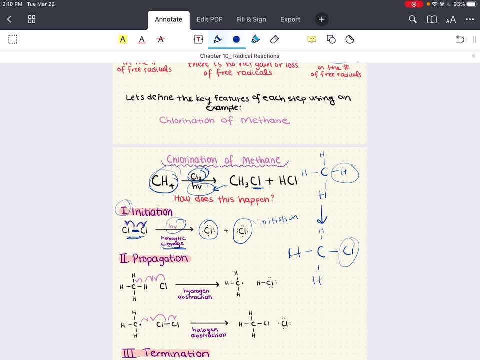 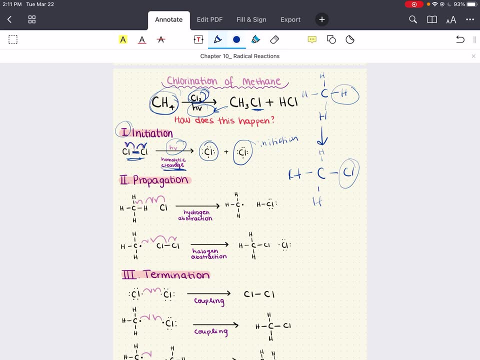 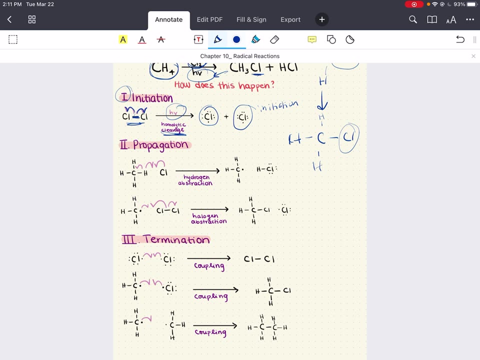 So now we have these chlorines, Chlorine radicals- Fantastic. Now that we've initiated a radical mechanism through homolytic cleavage, we can move on to the second phase of a radical mechanism, which is propagation. Propagation is responsible for the observed reaction. 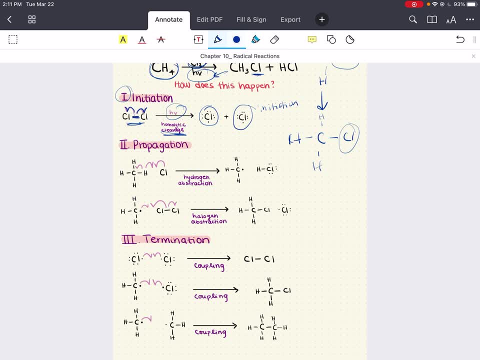 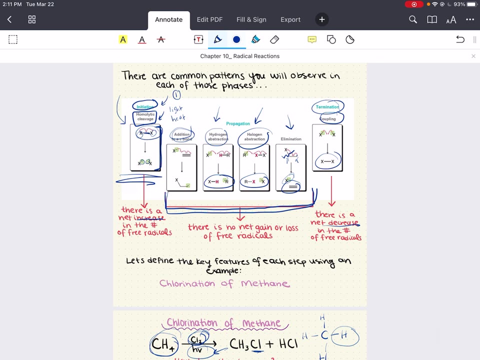 and the sum of each step is going to give the net reaction. That was that last note I made about propagation before we jumped into this example: Propagation, Propagation. You will see propagation. The patterns, the common patterns you'll see in propagation, remember, 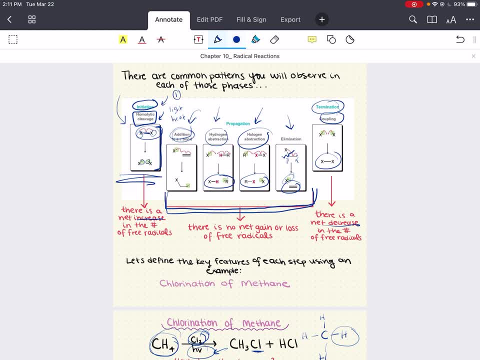 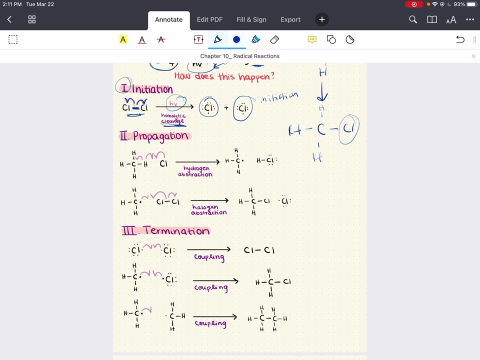 is either addition to a pi bond, hydrogen or halogen, abstraction and or elimination, And you can see a good mixture of any of these patterns during propagation. But at the end of the day, propagation is responsible for the observed reaction that we see here. all right, 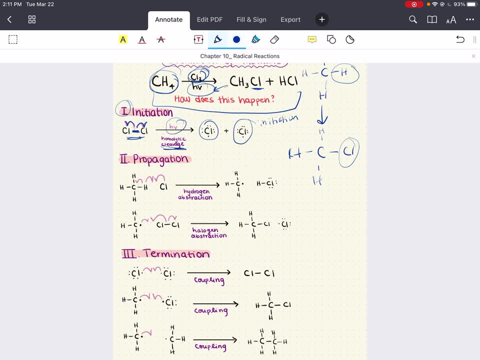 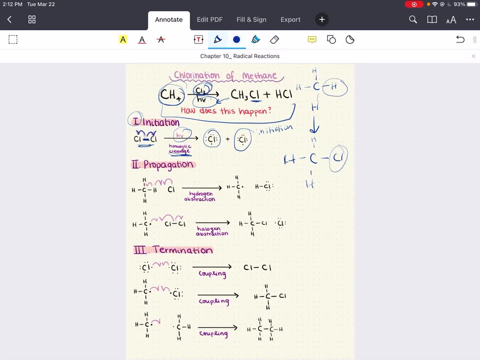 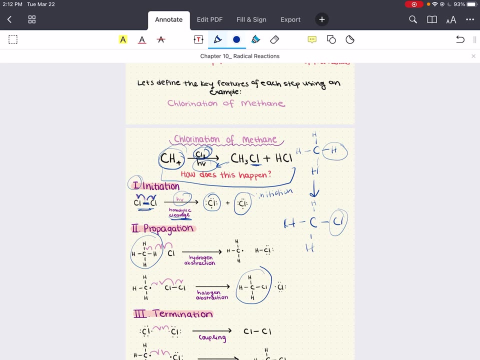 And the sum of each step that occurs in propagation is going to give the net reaction. So our ultimate reaction is that we want to take methane, convert it to this chloromethane group here. all right, So we start off with methane. 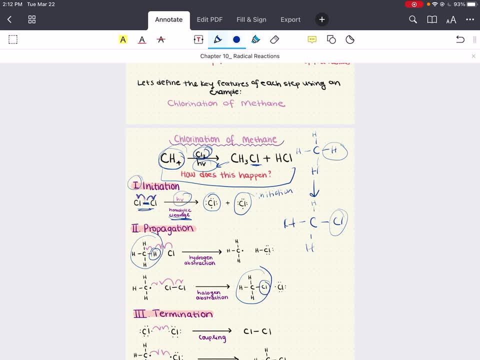 We are replacing one of the hydrogens with chlorine. That is ultimately what we're trying to do. So one of the first steps in propagation for chlorination of methane is hydrogen abstraction. Hydrogen abstraction here, a radical, this radical that we formed, this chlorine radical that we have formed. 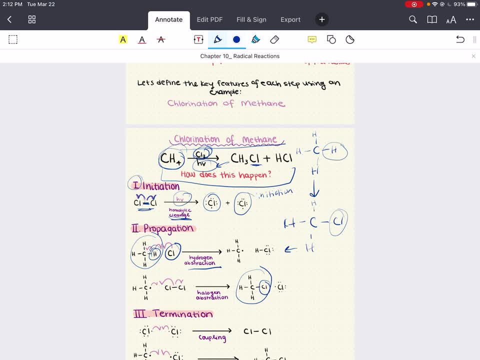 is going to abstract a hydrogen atom from our methane. So when our chlorine radical steals that hydrogen from our methane, we form methane, We form hydrochloric acid And now we have carbon with three hydrogens only and, of course, one single electron. 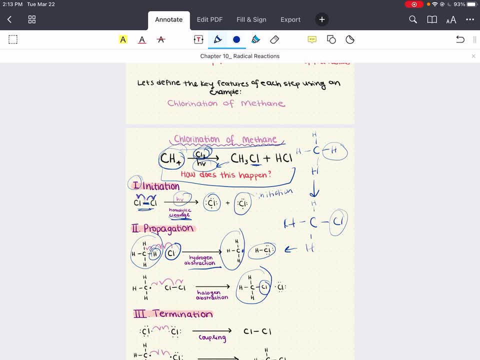 Now, what can happen is a halogen abstraction, all right. And now this radical that we formed, this methyl radical that we formed, it can abstract a halogen. It can abstract a halogen, The halogen, It can extract a halogen. 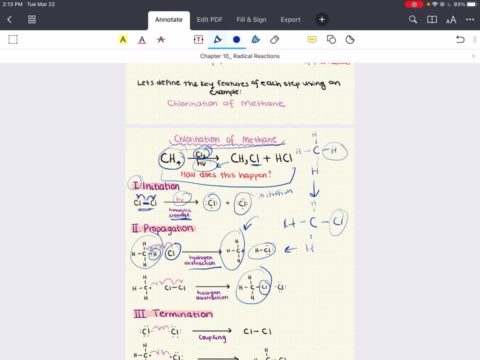 And it can extract a halogen, All right, And generate a new radical. So, with our Cl2 that we have, our methyl radical can steal one of the chlorines from our Cl2.. And what we form is the molecule that we want at the end of this. 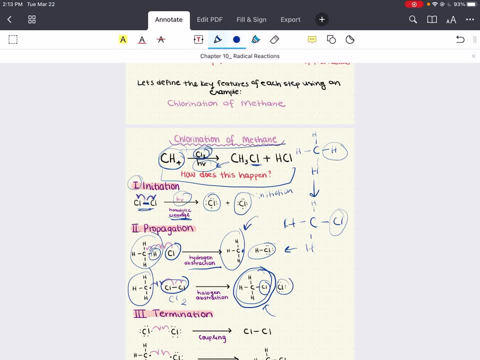 which is a carbon with three hydrogens and a chlorine, And again we have our chlorine radical here. Now, what were we saying about propagation? Well, propagation is responsible for the observed reaction, which means the sum of each step, and we have two here. the sum of each step gives the net reaction. So let's look at 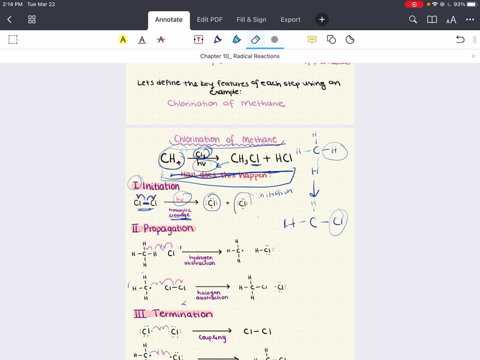 these two steps here, all right, and see what our ultimate net reaction is here. Well, in the hydrogen abstraction step, we have a chlorine radical in the reactants. all right, we have a chlorine radical in our reactants. In the second step, we have a chlorine. 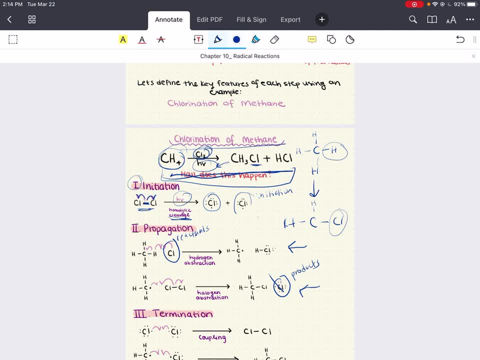 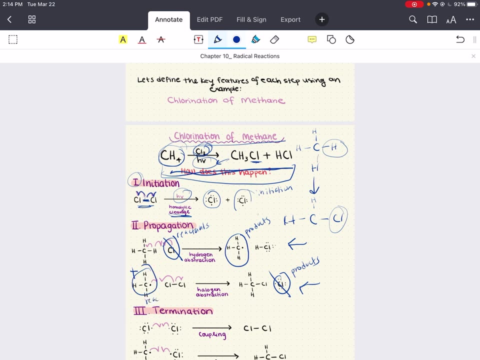 radical in the products. all right. so these cancel out whenever you add these two reactions together. Now we have a methyl radical in the products of our first step of propagation. we have it in as a reactants in the second step. When we add these two reactions together, that 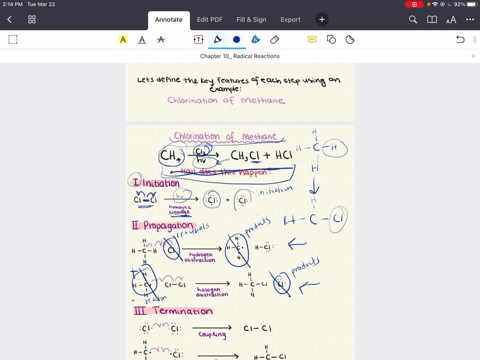 cancels out. Look what we have left in the end: In the reactants, we have our methane and our Cl2 when we add these two reactions, and in the products, we have our hydrochloric acid and our final product of chloromethane. in our products. That is exactly what we want ultimately, So 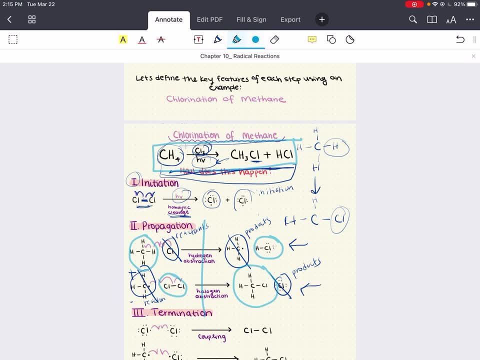 whenever you add these two reactions together you have a chlorine radical in the products of our writing up the propagation steps for a reaction. Make sure that the sum of each step when you add up all the propagation steps, all right, that at the end you get your net reaction all right. 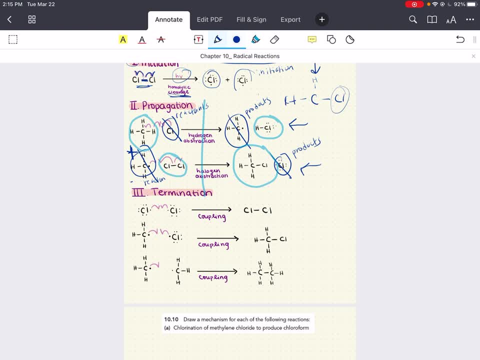 Now we can move on to our last final step, which is termination. This involves destroying radicals through coupling. all right, We see in the mechanism that we destroy the two radicals and we destroy the two radicals and we destroy the two radicals. 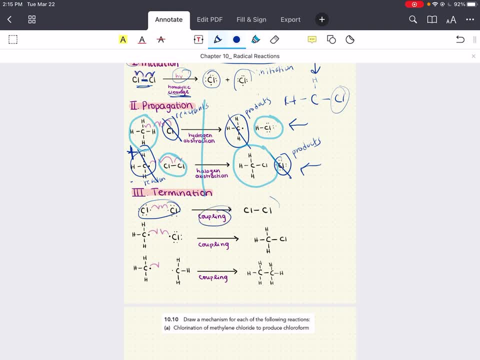 We destroy the two chlorine radicals, all right. They add up again through coupling. We destroy them, all right. What other kind of radicals did we have? Well, we destroy one methyl radical and one chlorine radical to get the final product we want. and also two methyls can, also two methyl. 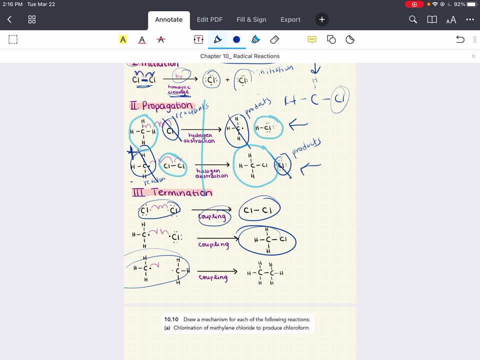 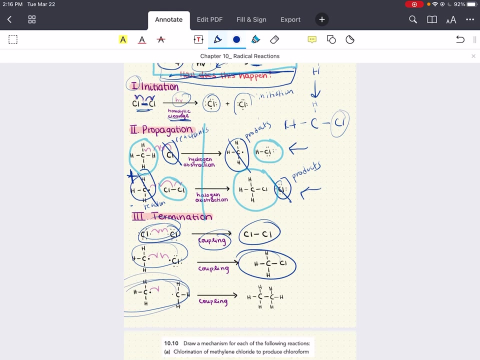 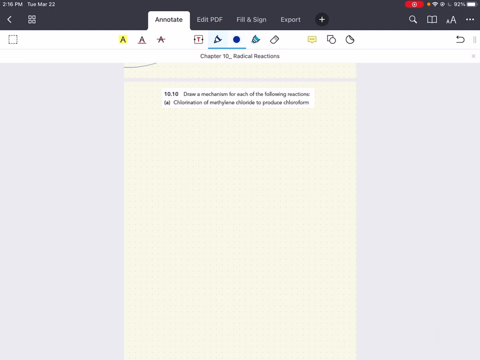 radicals can also couple and destroy that. You can destroy the last two methyl radicals as well. So your termination step essentially involves destroying radicals through coupling and they can react in several ways And this is the radical mechanism for chlorination of methane. Let's do a practice problem. Make sure we completely understand. 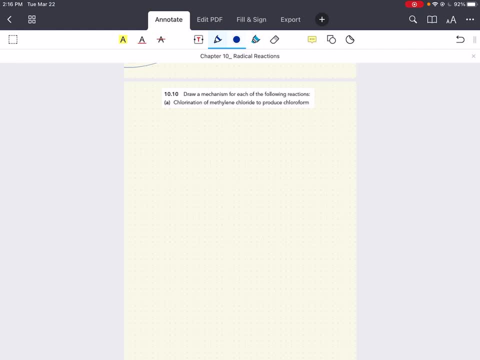 all the steps of radical mechanism. This question says: draw a mechanism for the following reaction: Chlorination of methylene chloride to produce chloroform. all right, So the mechanism's going to have three distinct stages. The first stage is going to be initiation. all right Here. 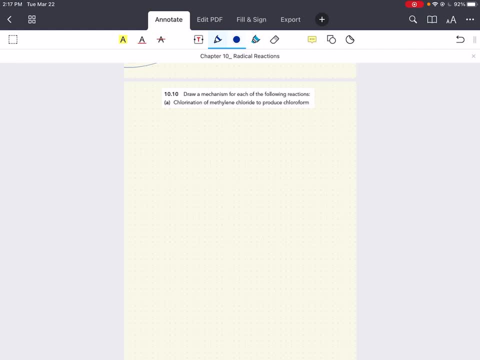 the chlorine bond is broken to generate chlorine radicals. This step is going to require two fish hook arrows, all right. Then there are two propagation steps, a hydrogen and a halogen abstraction, And then there's going to be our final step, our final phase, which is our termination. 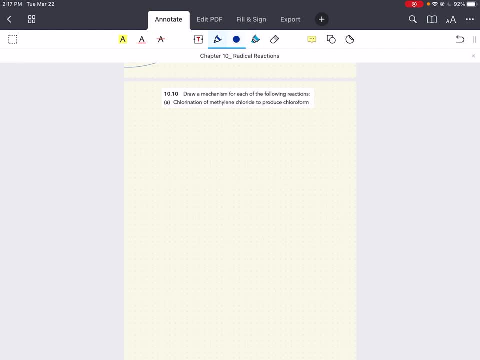 step. There's going to be a few, because there are many radicals that we've formed. We're going to couple them together and ultimately destroy our radicals. So let's go ahead and draw this mechanism. Chlorination of methylene chloride: So let's go ahead and draw this. Methylene chloride looks like a carbon with two chlorines. 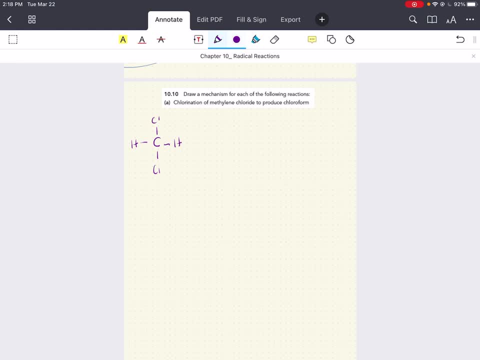 all right. Chloroform is going to look like carbon with three chlorines- Chlorines- attached to it, all right, And we're going to treat this with Cl2 and, of course, some light. all right. So we're going to go from methylene chloride to chloroform through. 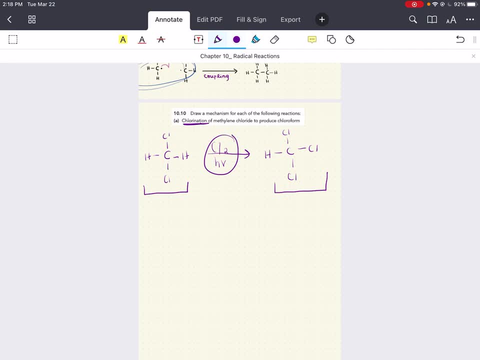 chlorination, which means using Cl2 and light or heat. all right, Now I talked to you through the steps. We're going to actually draw them out. all right, Your first step is initiation. Initiation involves homolysis. 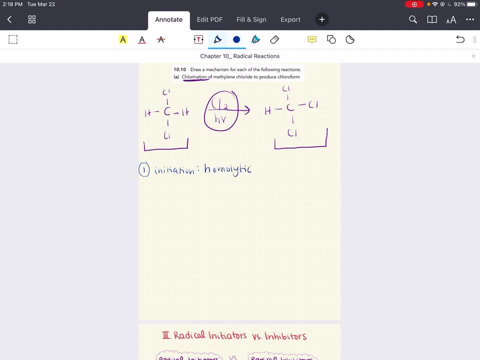 Homolytic cleavage. Homolytic cleavage, specifically, of your Cl2.. What's going to happen here is each chlorine gets one electron. This is initiated through light or heat, And what you get are two chlorine radicals as a consequence of homolytic cleavage of Cl2 initiated by light or heat. 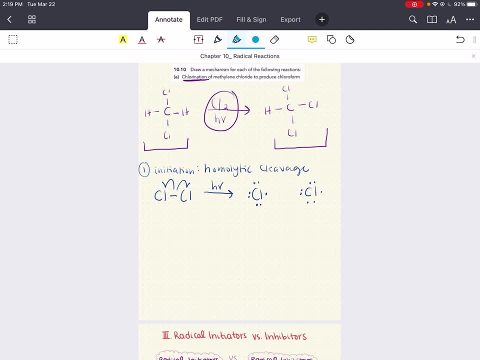 Fantastic. That's our first step, initiation. Now we move on to our second step. Our second step in a radical mechanism is propagation, Propagation. all right, Here in propagation, remember, this is going to be the steps that are responsible for our total observed reaction. That means the sum of each step that happens. 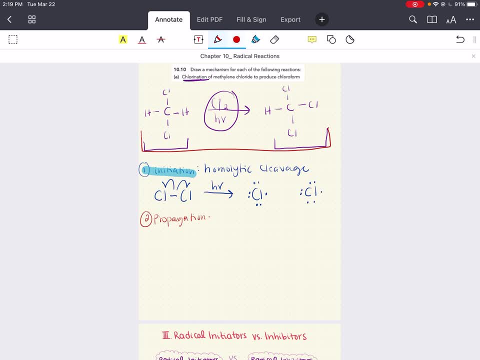 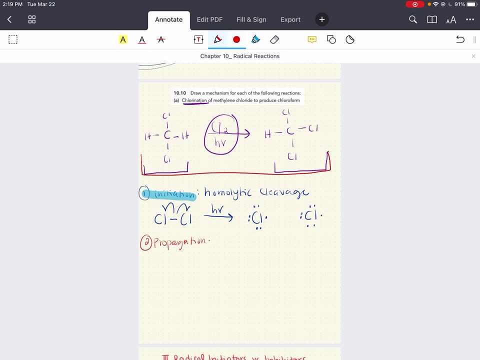 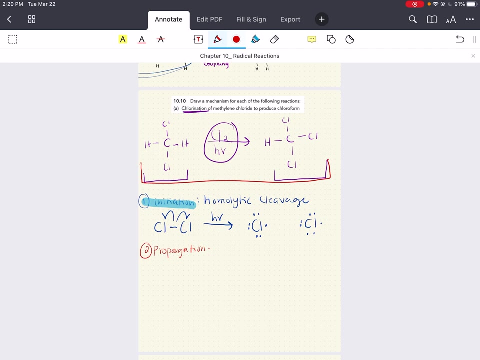 gives the net reaction. Now, this is still a chlorination mechanism, So it's going to follow very similar steps to what we saw for chlorination of methane. This will still abide by the same steps we saw in that example. So for chlorination of methylene chloride to 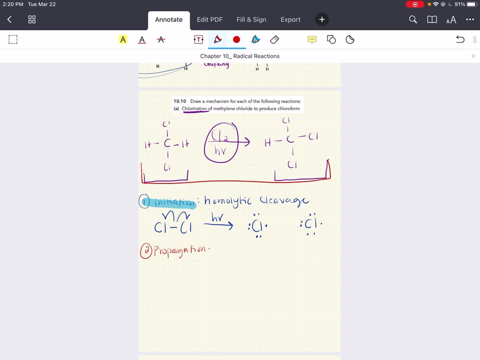 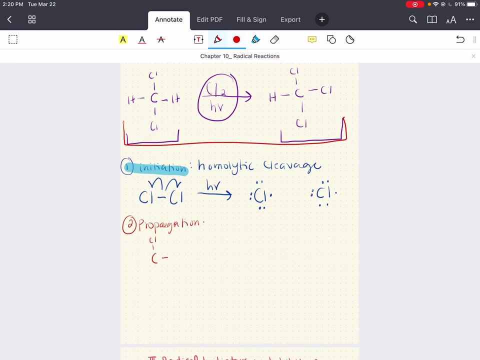 chloroform. we are also in the mechanism going to see for the propagation step: hydrogen, hydrogen abstraction and halogen abstraction. So we're going to go ahead and we're going to draw that All right Now, starting with starting with methylene chloride. 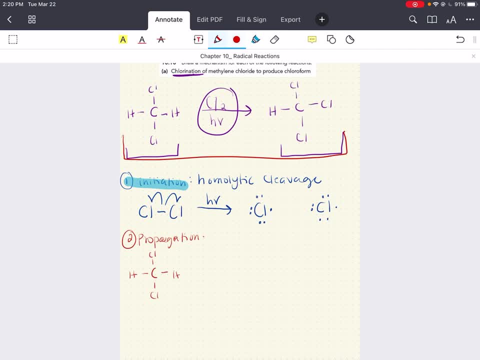 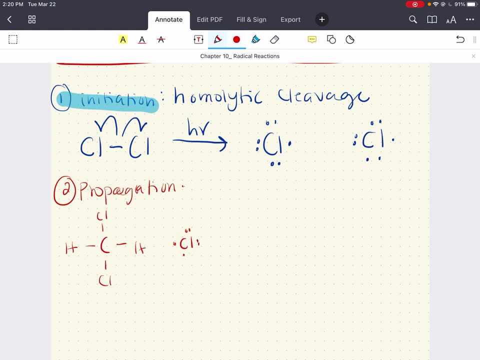 All right, Our first step is going to be hydrogen abstraction. All right, So our chlorine radical and the hydrogen of our methylene chloride- All right, They're going to form a bond. So we're going to take one of the electrons of our radical and one of the electrons for this bond. 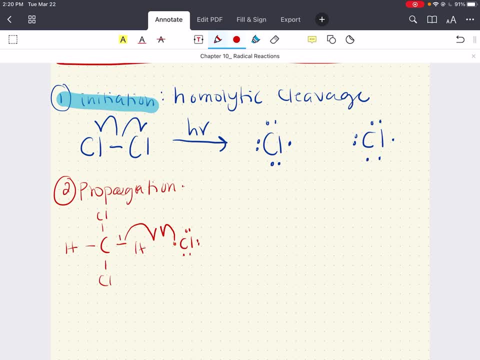 between carbon and hydrogen, All right. And that means that the other electron gets left behind. for the carbon, What we get is a radical- All right, This radical right here- and hydrochloric acid. This is for hydrogen abstraction, All right. The next step is: 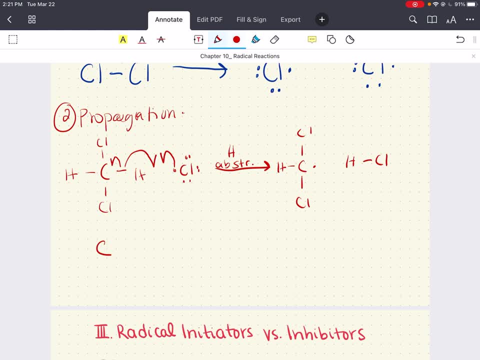 halogen, Halogen abstraction. So we take this radical that we formed in our last step and it can react with Cl2 that we had to begin with. Now this electron from the carbon and a single electron from the chlorine chlorine bond are going to form a new bond between this carbon and chlorine, And this 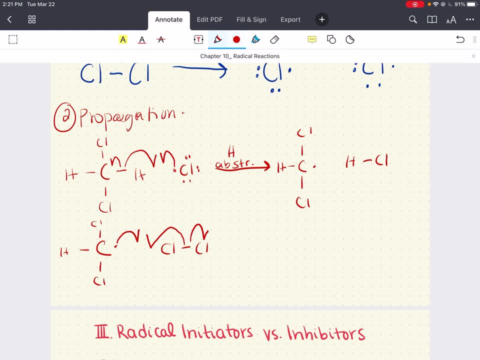 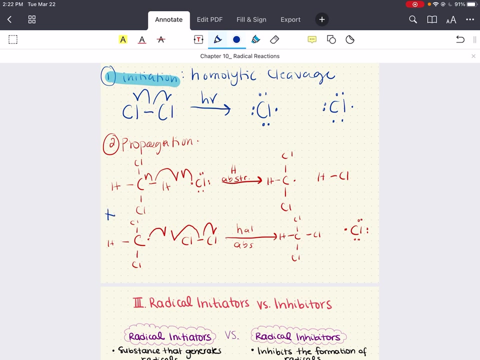 last electron from the bond gets left behind to the chlorine. All right, This is halogen abstraction. What we get here is our chloroform- All right, What we get is our chloroform and a chlorine radical- Fantastic. Now let's look at the net reaction of these two steps. If we added both of these steps, 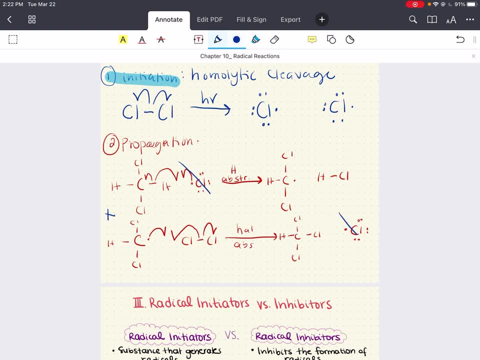 Well, in one step we have chlorine in the reactants and chlorine in the products. When you add these two reactions together, those cancel out Fantastic. Now we have this radical in the products of one and as the reactants of another, And so those cancel out What we are left. 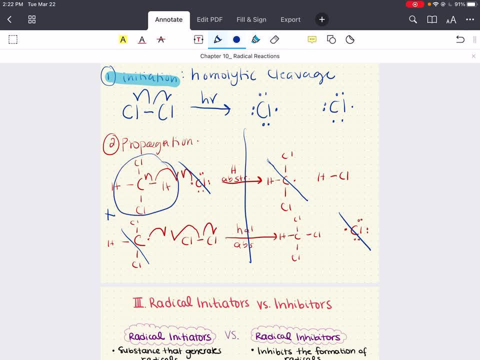 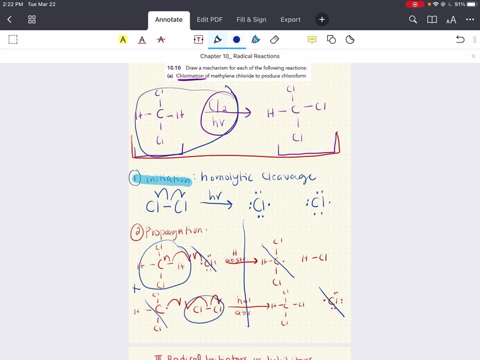 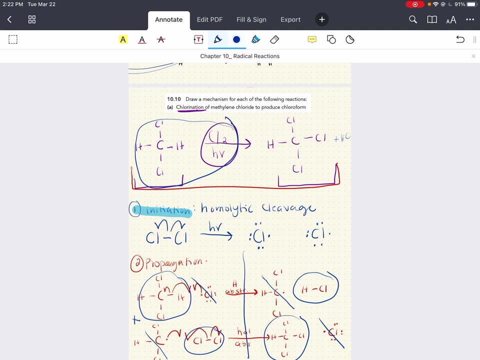 with in the reactant side. then is the methylene chloride. We started off with NCl2, this part of the reaction, And for our products we have our chloroform and hydrochloric acid, All right, Which is this part of the reaction. That's fantastic. That's exactly. 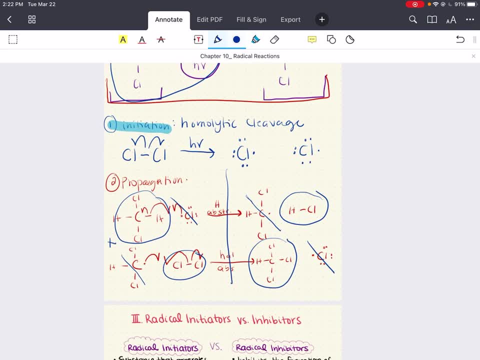 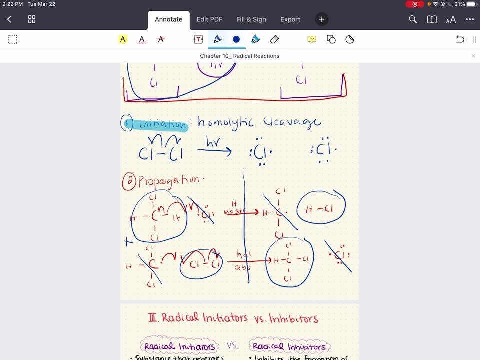 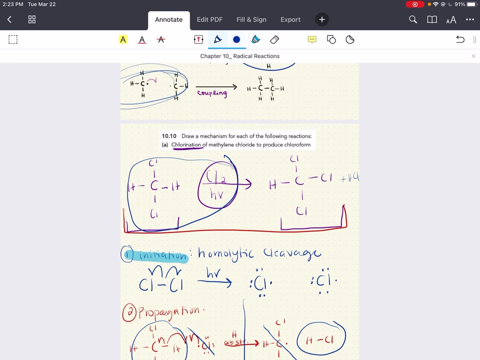 What we wanted to get. This is the net reaction we're looking for, So we've appropriately written the propagation steps for this reaction. Now, last but not least, is termination. All right, So now your radicals can be coupled together to destroy each other, All right, And so we have no room. 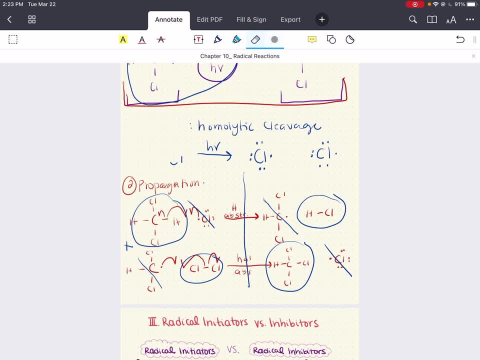 here. I'm just going to erase our initiation and write our termination here. All right, So our last step is termination, And so our radicals can couple together to destroy each other. So two chlorine radicals can react with each other Like we saw in our example here. All right, 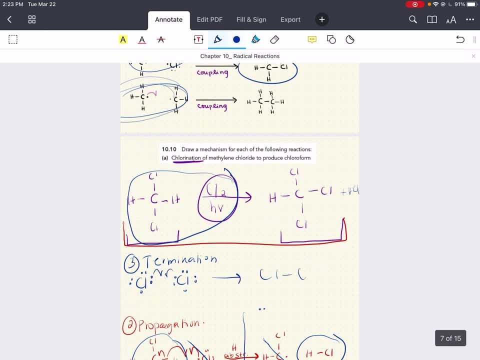 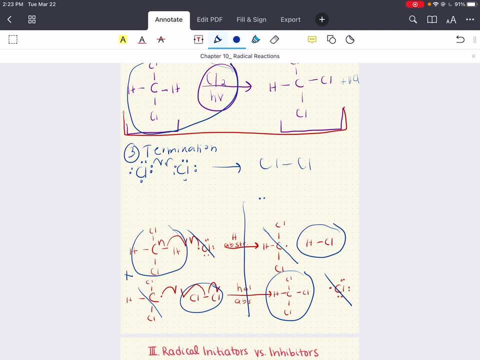 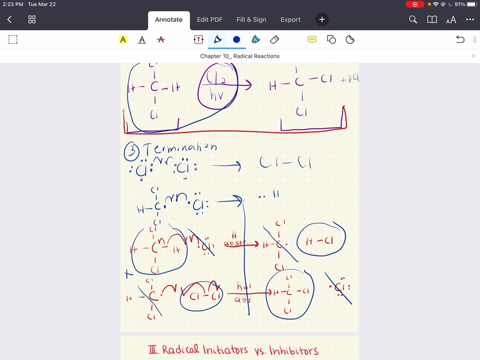 They can couple to form Cl2.. Also, we can couple our. There's no room here. We can also couple ClH, This radical that we formed in our propagation step, with a chlorine radical. Ultimately all right to form our chloroform and thereby destroying more radicals in our 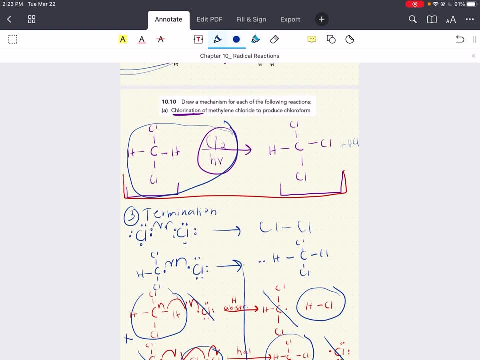 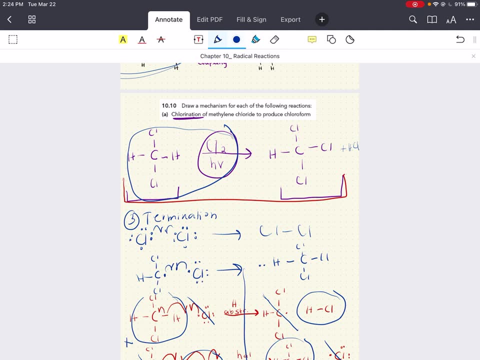 termination step: Fantastic, All right. That is all for today. Next time we're going to go ahead and finish the rest of chapter 10.. If you have any questions, leave them in the comments or reach out to me personally. I'd be more than happy to help If you want to see more practice problems. 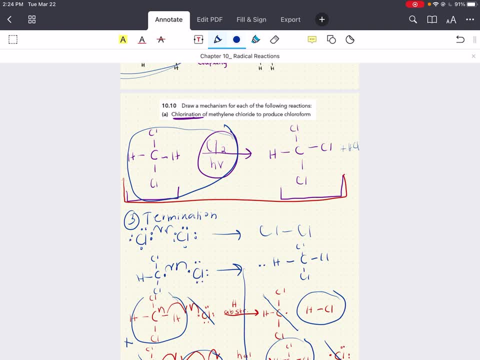 for the next chapter. I'll be happy to help you, So if you have any questions, leave them in the topics that we've covered today. Let me know. I'd be more than happy to accommodate that. Other than that, good luck, happy studying and have a beautiful day.